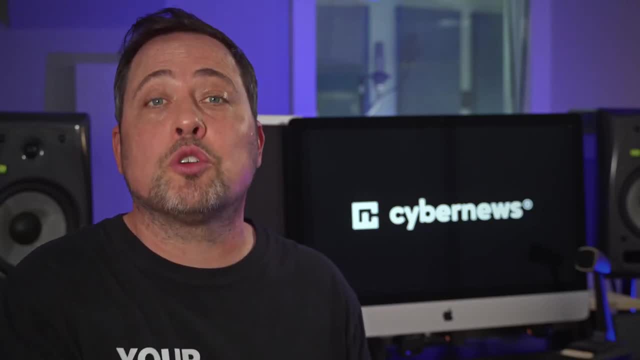 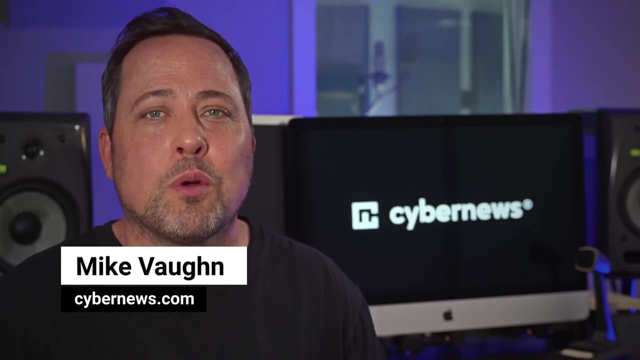 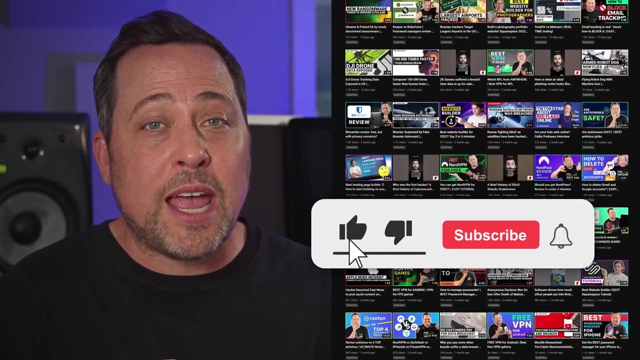 Maybe it's actually a good time to drop a little friendly reminder to ensure that everything connected in your world is protected. And welcome to CyberNews. I'm Mike here with my regular Cybersecurity 101 content: Easy to understand tutorials and reviews, alongside reliable news and online privacy tips. 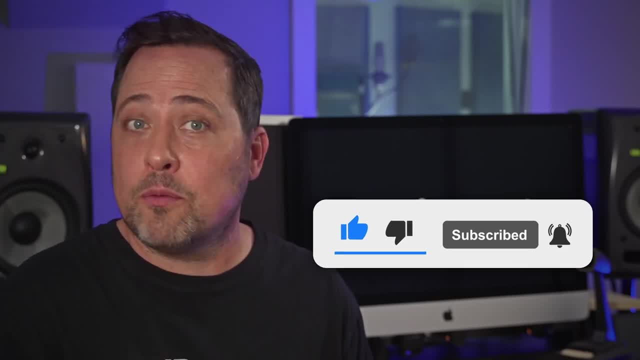 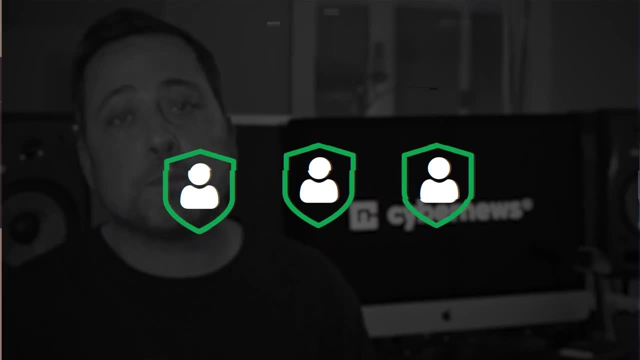 You know you should probably just go ahead and subscribe to the channel so you never miss another video. just saying Now: protecting all of your online accounts and your precious data has never been more important, especially during Cybersecurity Awareness Month 2022.. 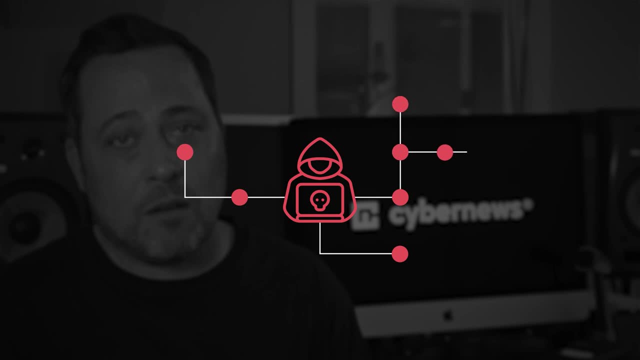 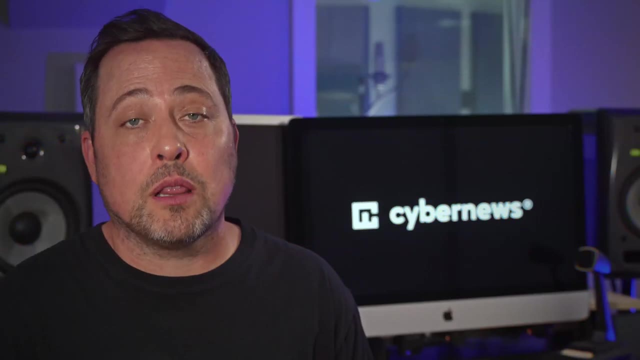 You see, cybercriminals are perfecting their tactics every year, And with that, you should be looking at ways of protecting yourself as well. I mean, this year alone saw a bunch of colossal breaches and leaks, And looking forward to 2023, yeah. 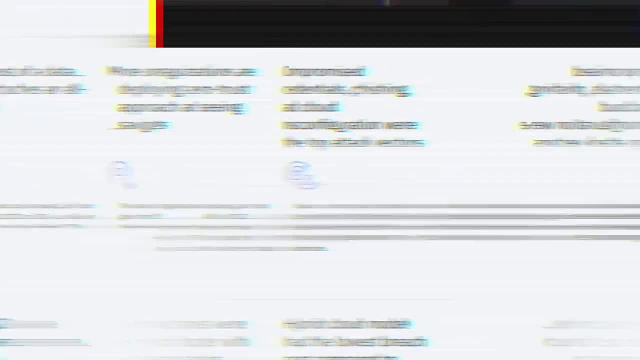 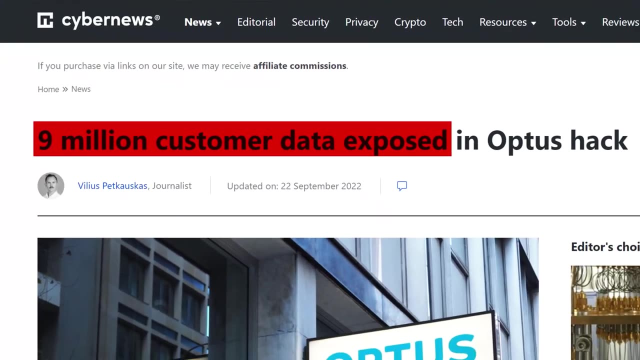 it does not look like things are gonna be any different From scraping 500 million LinkedIn users' data and then selling it online to 9 million customers' data being exposed. yeah, businesses and individuals are learning the importance of cybersecurity the hard way. 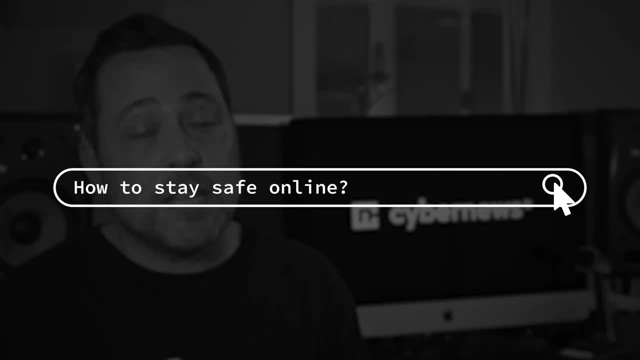 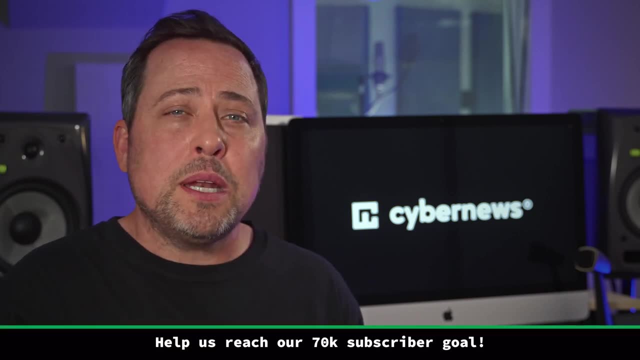 Okay, so how to stay safe online? Well, as an individual, there are various threats to look out for, So I'm gonna run through some of the more prevalent ones real quick. A common attack vector for cybercriminals is spam emails or phishing attacks. 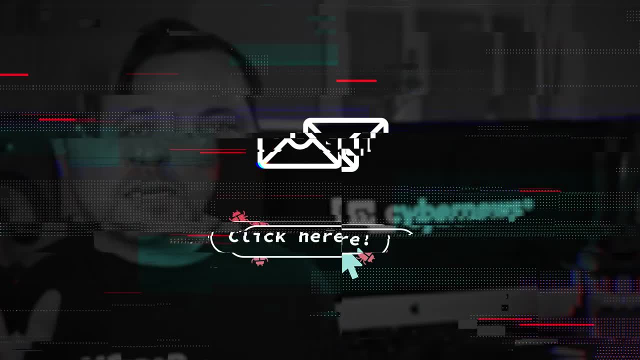 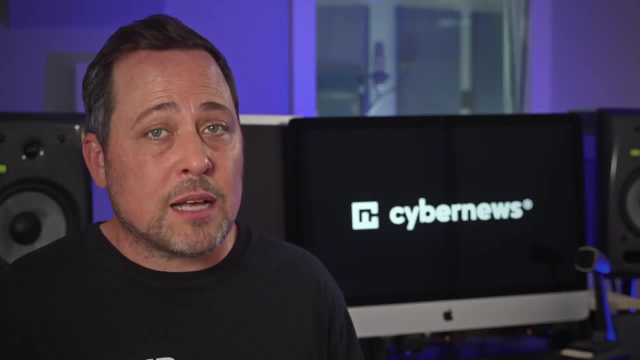 This means you click a link in an email and bam, you got Trojan, spyware or ransomware- it's all deployed right there on your device. Many victims have lost access to not only their devices but their prized data through these types of attacks. 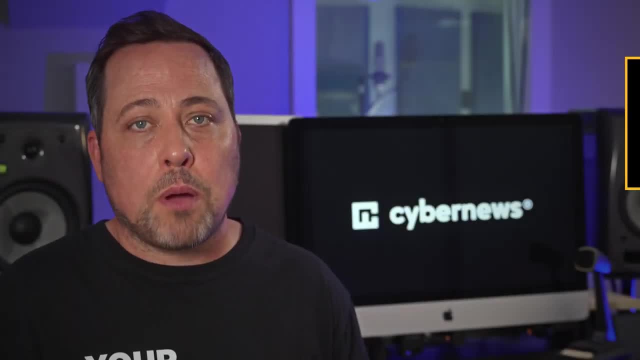 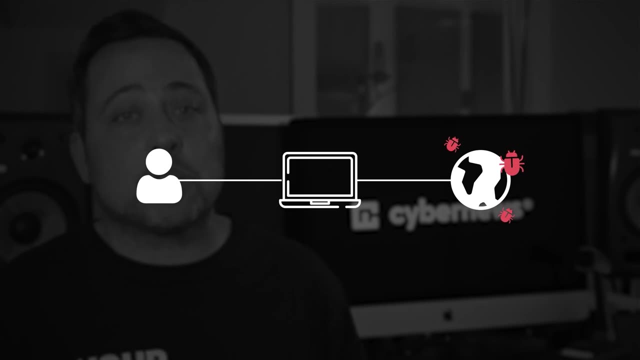 Third-party ads are also a culprit. You know the ones that pop up on the side as you browse and then, once clicked, they can often redirect you to malicious sites or sometimes just directly infect your computer with malware. Then there are DDoS attacks and general hacking. 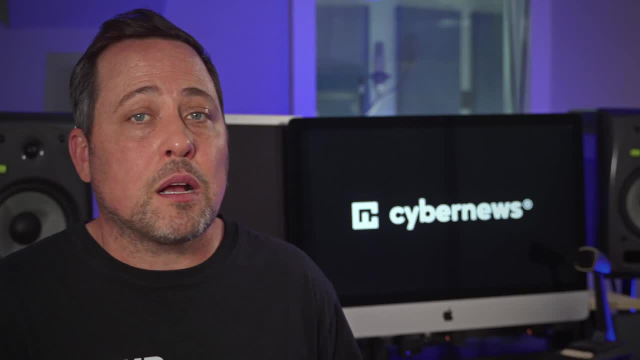 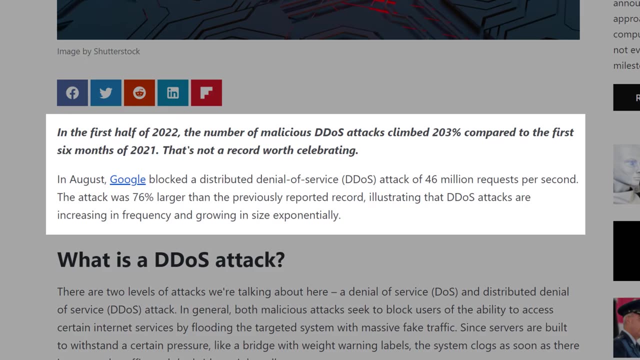 Despite usually targeting businesses, DDoS attacks are usually targeted at businesses and the most common cause of DDoS attacks is the lack of data. DDoS attacks climb 203% in the first half of 2021, and generally malicious actors will gain unauthorized access. 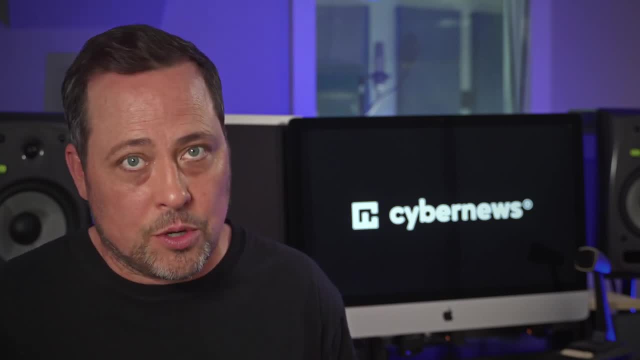 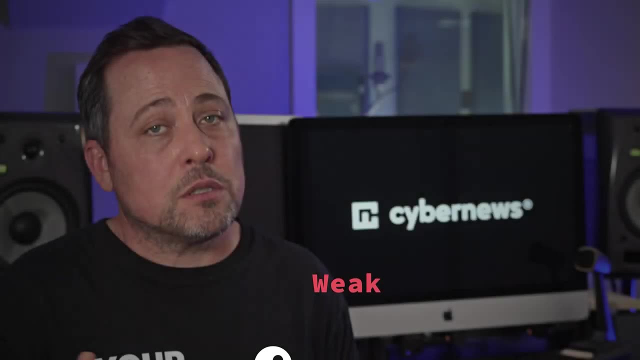 to your device through a vulnerability and then steal your data. This can sometimes happen because you've used a weak or reused password across various accounts, which is a total no-go and a piece of cybersecurity advice that many experts already warn you about right. 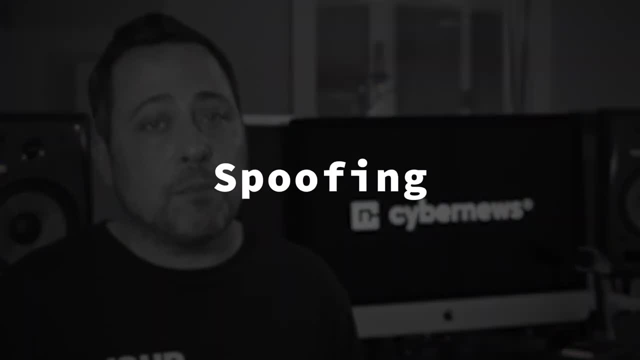 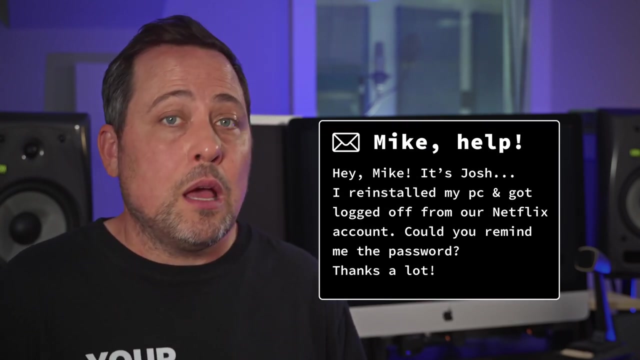 You know who you are, Then phishing and spoofing are something you should look out for. Basically, they're about luring the victim to give up personal information themselves, Like, say, you receive an email, supposedly from a colleague, asking for company information or a password that they've misplaced. 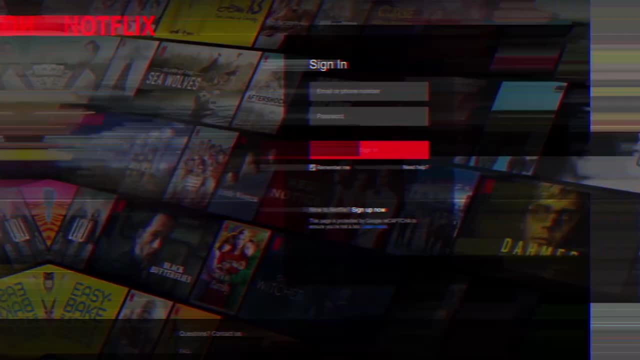 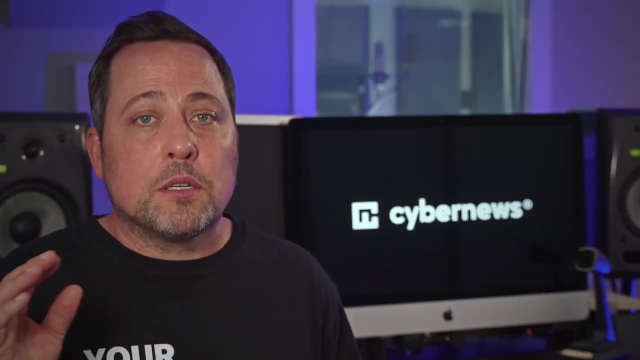 a Facebook message from a friend, or maybe you've opened up a spoof version of your favorite website. You know, maybe you did it by accident, who knows? But they all have one purpose: to trick you into offering up sensitive information, be it banking credentials, email addresses. 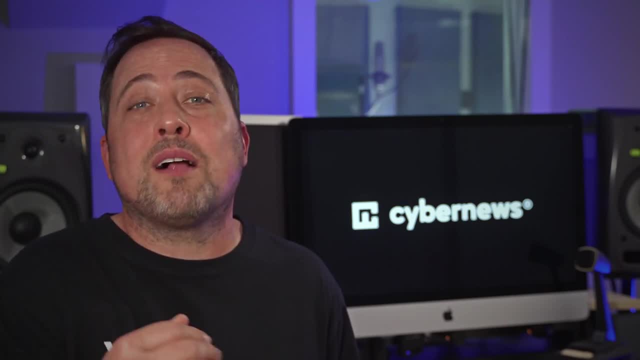 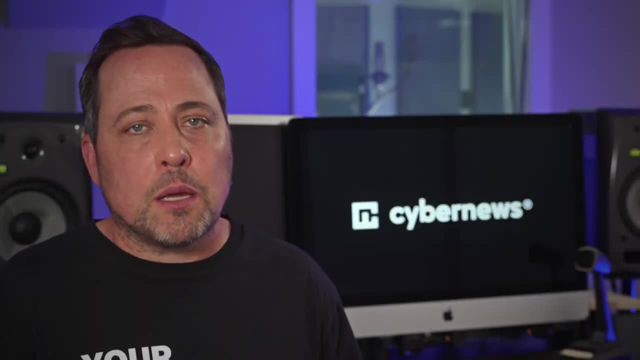 or whatever else the cybercriminal needs to create a profile emulating you. Now another area that's often overlooked: Wi-Fi eavesdropping. I get it. desperate times call for desperate measures, and we all need to jump on Wi-Fi real fast. 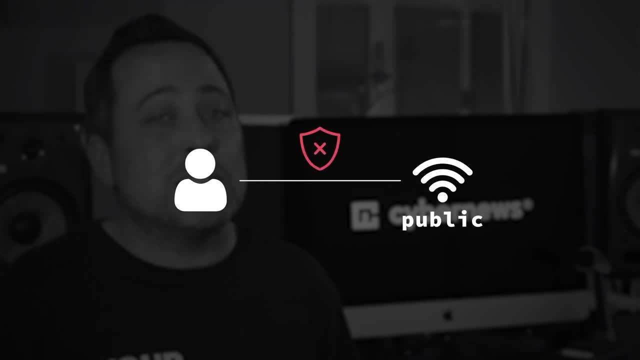 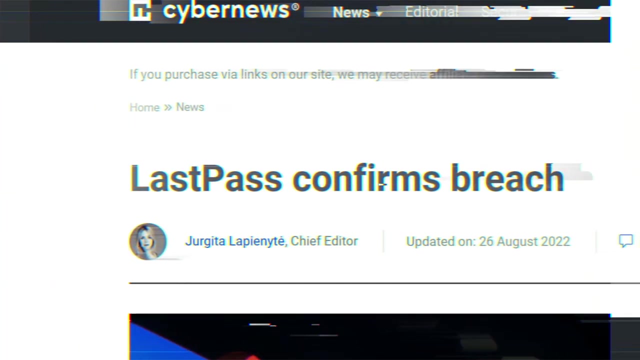 but using public Wi-Fi means your connection is unsecured, meaning a cybercriminal could eavesdrop on your online communications or, worse off, gain access to your system altogether. And you see, the consequences of not having cybersecurity products and choosing the wrong ones are grave. 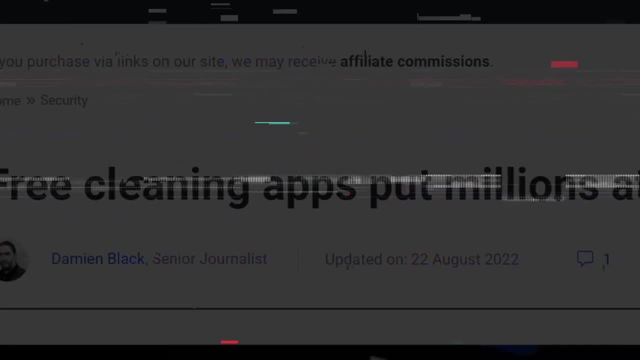 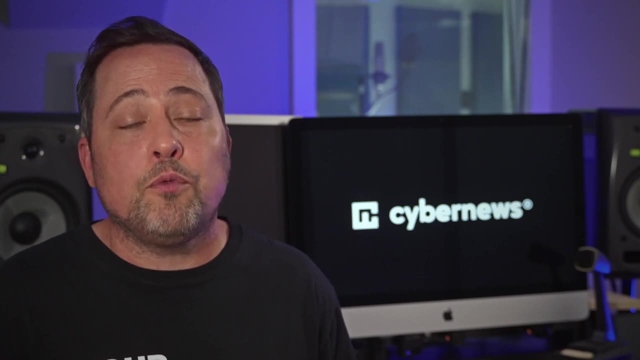 with untold companies storing sensitive data without proper protection. Now, that's why I'll run through some online privacy and security tools that you should get this year if you want to avoid falling prey to a cybercriminal. But first a little quick side note. 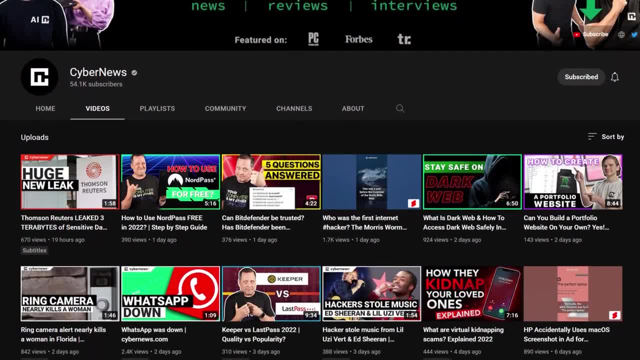 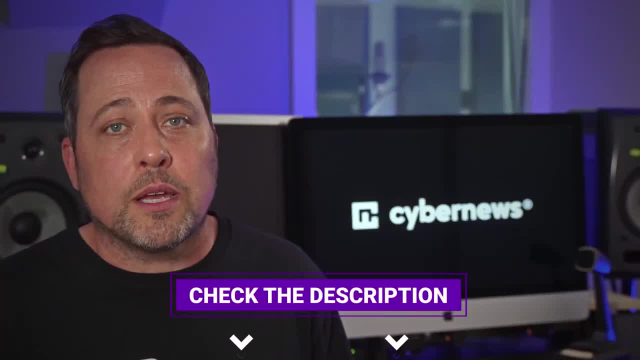 if you need specific provider recommendations after this online privacy guide, explore our channel. We probably have it. We've got a lot of in-depth reviews, along with exclusive discount links that we usually put in the video description, Just saying you might want to look there. 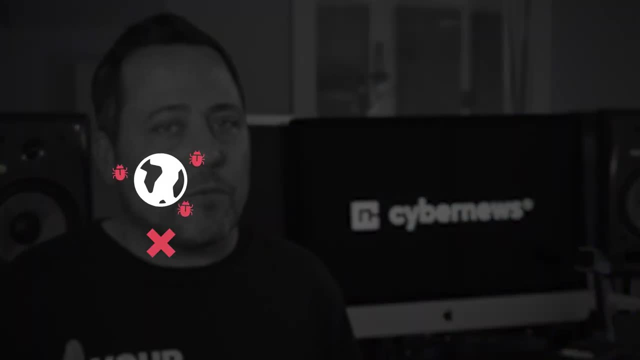 Okay now, if you want to avoid suspicious websites that could infect your device, leak your banking credentials across the web, or if you just want to protect all of your devices in real time, well then an antivirus is a must, And generally a lot of the free ones. 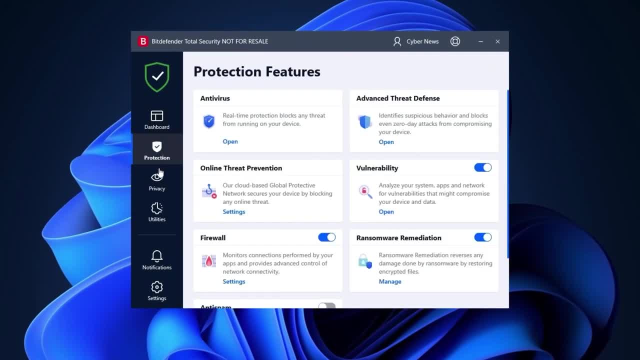 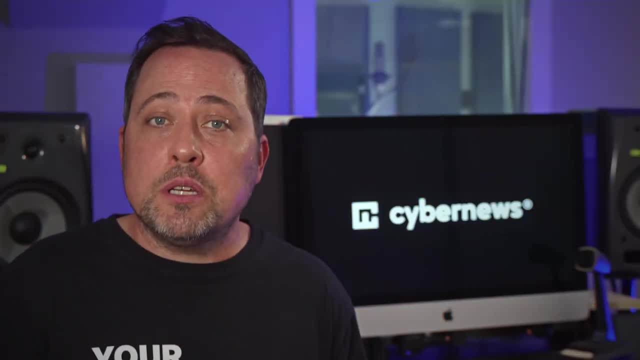 won't have the real-time protection or the strong firewalls that you need. So you need to be sure to do your research and get the stuff that works for you And if you're looking for a way to protect your device and, as we mentioned, online tracking by your ISP. 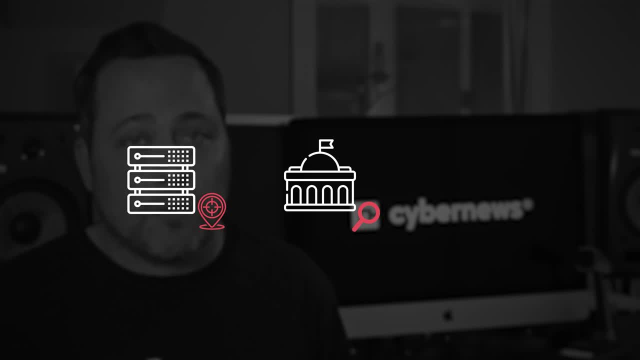 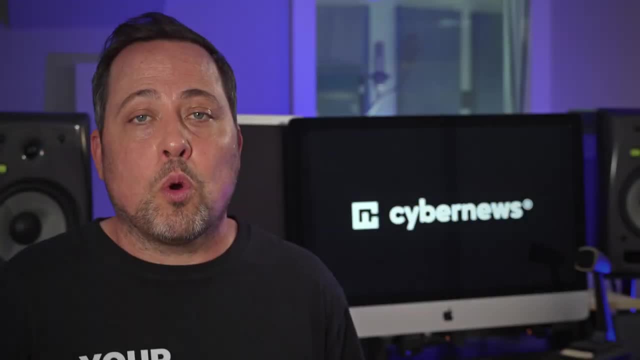 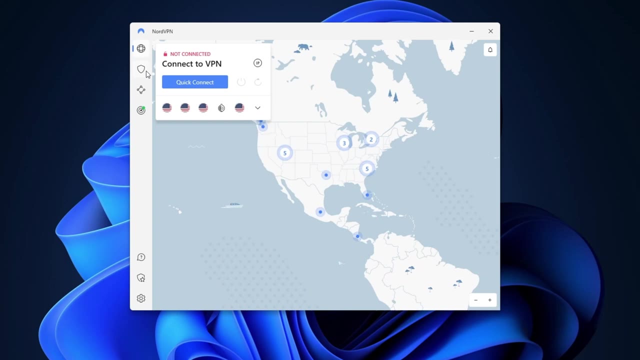 your government or whoever, is a serious threat to your privacy, And the dangers of public wifi can be avoided with a reputable VPN provider. There are even more advantages to using a VPN, but a reputable VPN is the answer to how to protect your online data. 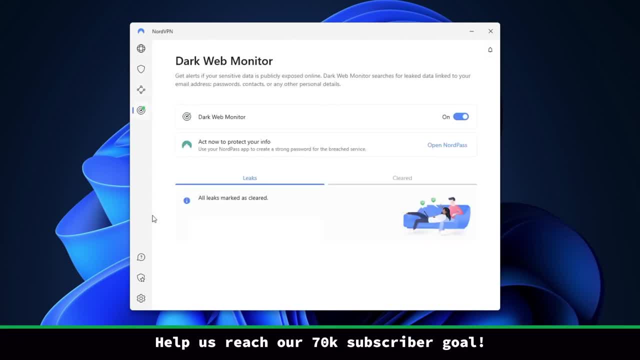 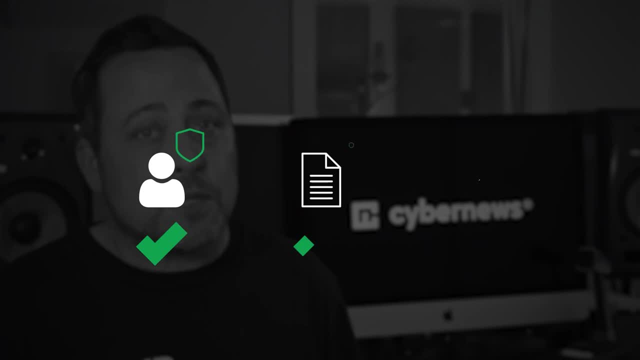 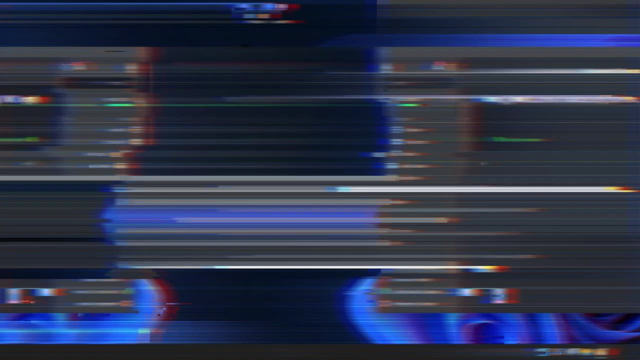 It secures your connection by using encryption and making it nearly impossible for a cybercriminal to intercept your connection. And if you're looking to secure all of your online accounts and their data, one of the most recommended tools is a trustworthy password manager. These not only store passwords. 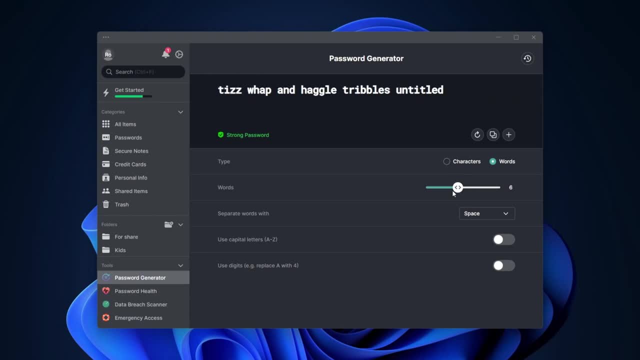 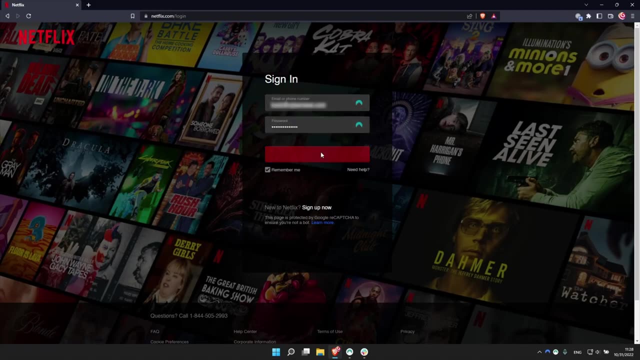 but they can generate really good ones too, And they make the whole account login process more secure and way more streamlined. A lot of password managers can also alert you if your credentials end up on the dark web, and some can even let you securely send passwords. 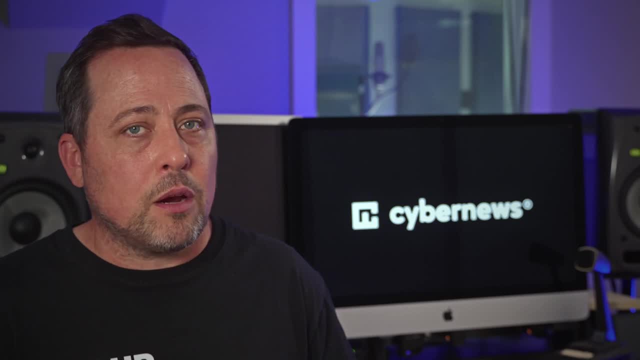 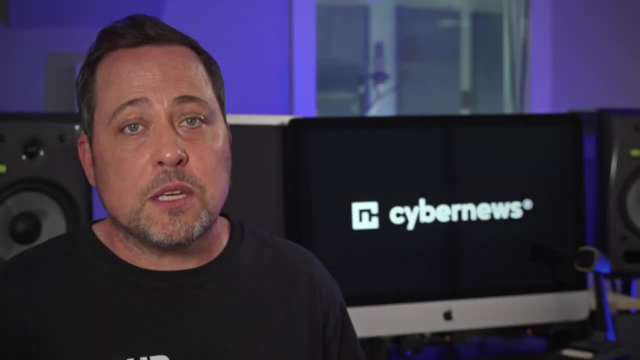 when you need to. Now for the true privacy seekers out there who might be looking to avoid a VPN, you should consider an anonymous browser or even an anonymous email service. That's gonna help maximize your anonymity as you browse and register your online accounts. 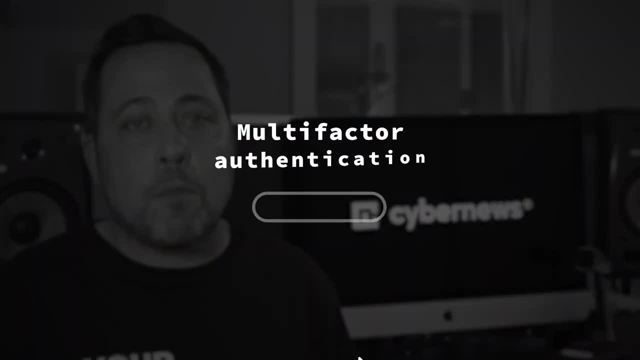 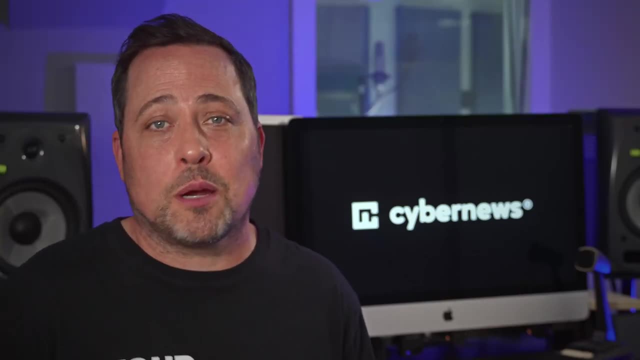 Oh, and also, you should also enable 2FA or MFA, multi-factor authentication on all of your relevant accounts. Okay so, look, this is just a quick introduction to cybersecurity, and I cannot tell you that every tool on the market is worth your hard-earned. 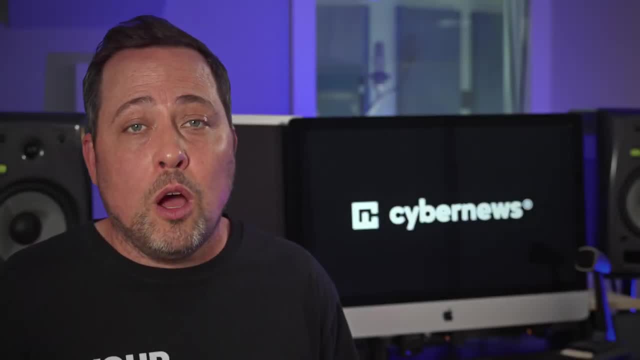 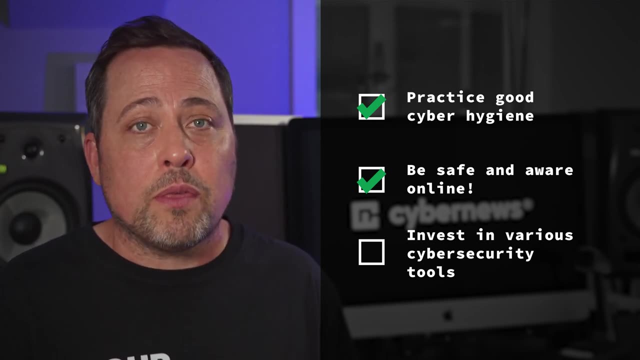 dollar and heck. I can't even say that just one tool alone could be a one-time be-all fix. So please be sure to practice good cyber hygiene to begin with and then keep your eyes peeled for anything suspicious And, when you're ready, invest in various tools. 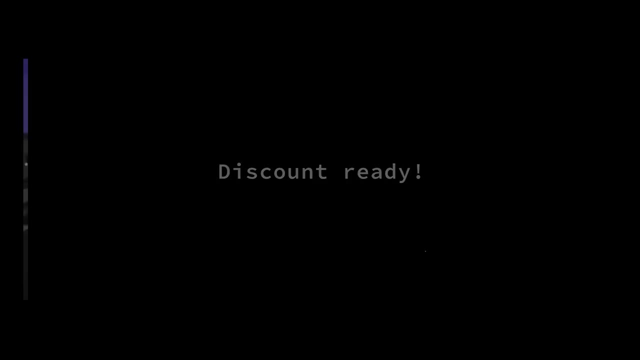 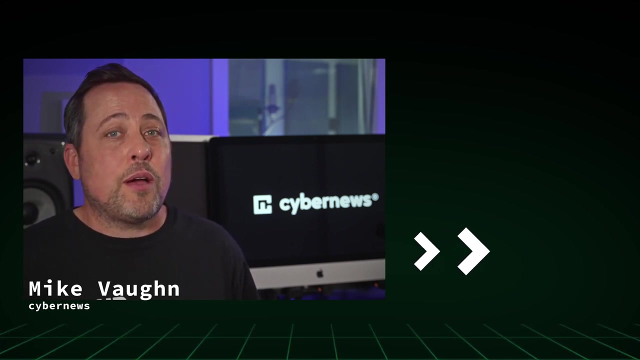 that work in conjunction with each other for the best chance of safeguarding all aspects of your digital life. All right, have you tried any of my recommended tools here? Do you have any national cybersecurity awareness tips? Let's hear them. Go explore more of our thoughtful content.